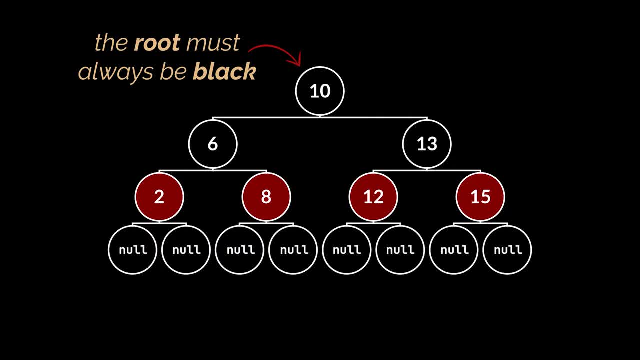 color. So, as I was saying, the root node must always be black, and null nodes, like the ones you see at the bottom of this tree, are considered black too. Every node starts off as a red node when it is created or inserted into the tree and on top of this, the parent and children 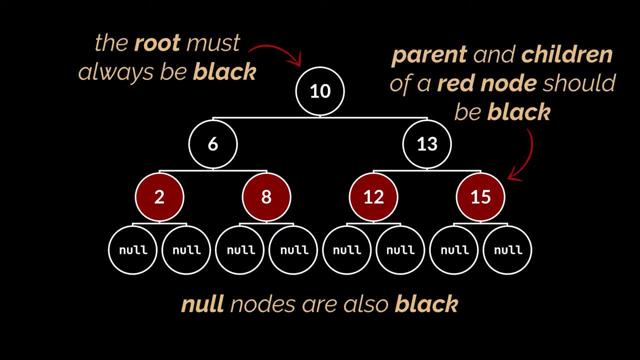 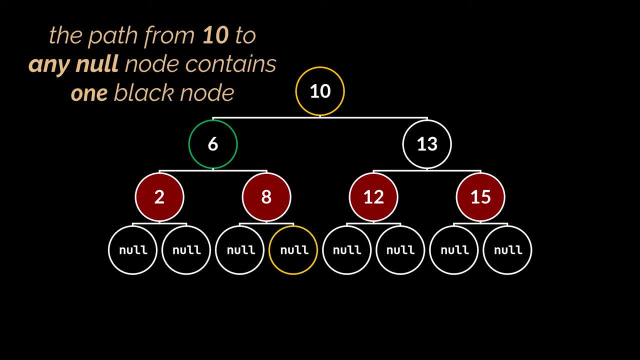 of every red node should be black nodes. And finally, if we try to draw the path from one node to any of its null descendants, all these paths should contain the same number of nodes. Okay, I know it's a lot of conditions, but, trust me, every single one has a purpose. 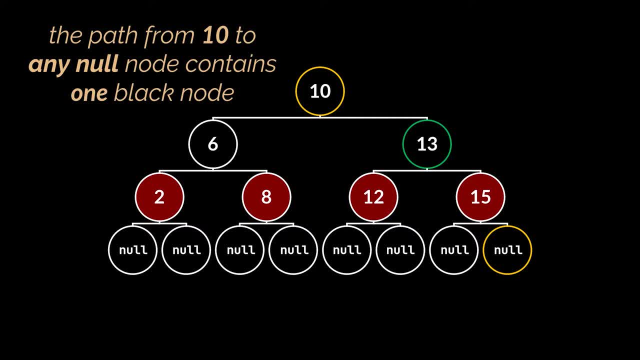 What purpose? Why should we have a black parent and a black child for every red node, and why the count of black nodes should be equal between a given node and all of its null descendants? Take this tree as an example. Now, practically you may not encounter such a tree in your 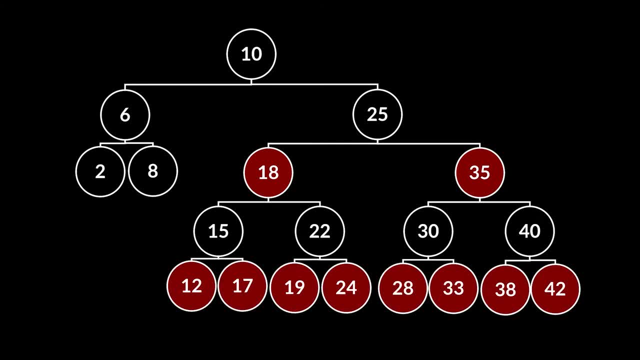 applications. However, if you take a closer look, you will see that all the conditions we just stated are respected. The root is black, The black and the red nodes are equal. So if you take a closer look, you will see that all the conditions we just stated are. 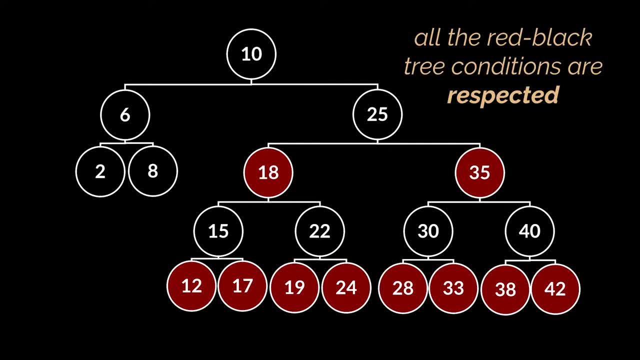 respected. The root is black. The black and the red nodes are equal. The black and the red nodes count from the root node to all its null descendants is equal- in this case it is two- And all red nodes have black parents and children. 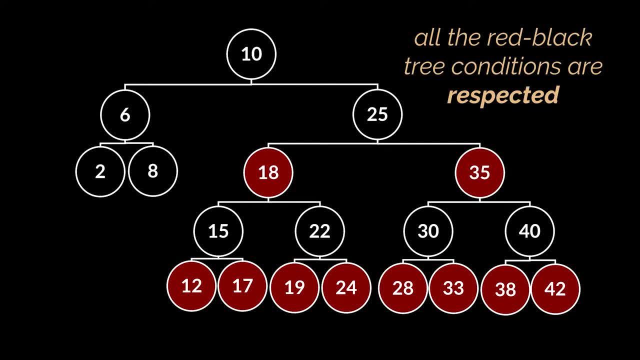 But, as you can see, this tree is not quite balanced. Well, what you see in front of you is one worst-case scenario. your red-black tree can reach a threshold which is, on one side, a complete set of black nodes and, on the other, an alternating red-black variation. 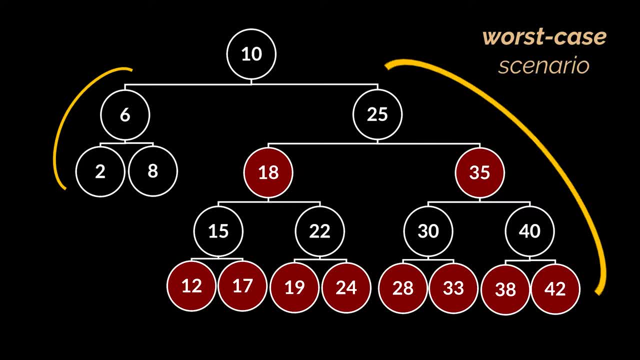 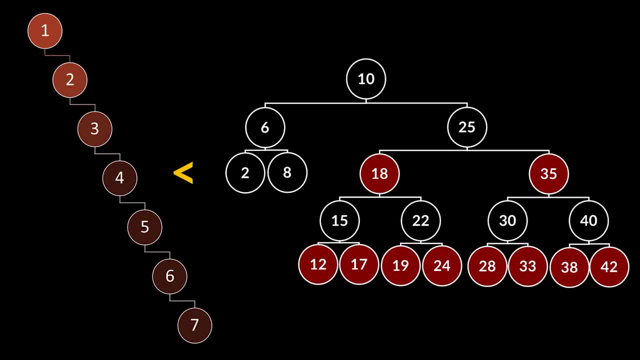 However, even like this, this tree is still way better than your simple binary search tree. The tree we have here is not quite balanced- not completely, but it is kind of balanced and surely will still perform better than the worst binary search tree we can have Now if you had used the AVL tree implementation. 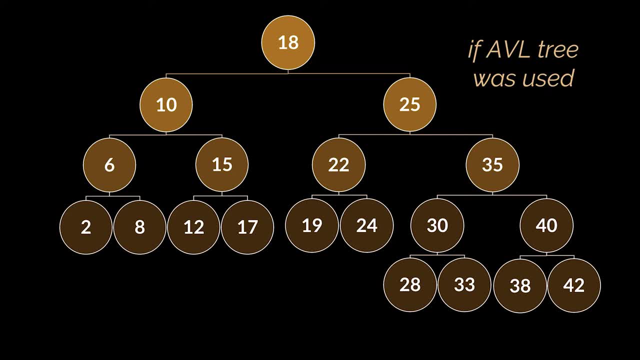 it would have looked something like this. But here we have to ask the question: are these extra rotations worth the time they are taking? You see, to reach this state we had to do way more than one simple rotation, and, in some cases, the time taken by these 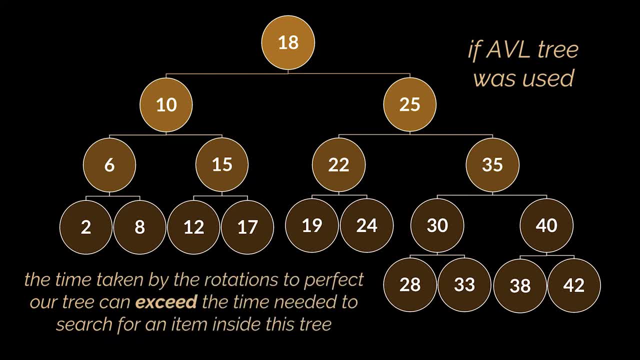 rotations to perfect our tree can exceed the actual time we need to search for the item in a not perfectly balanced tree like the red-black tree one. So that is why red-black trees were born: to take the best of both worlds- not too many. 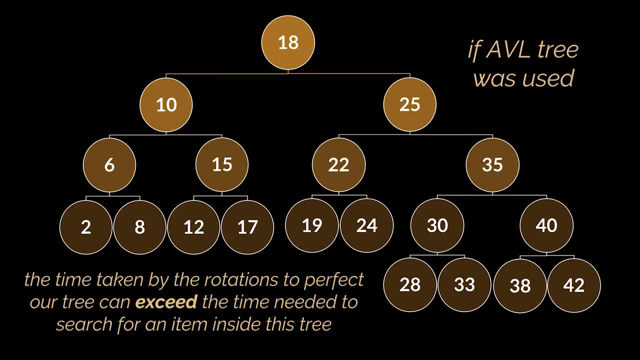 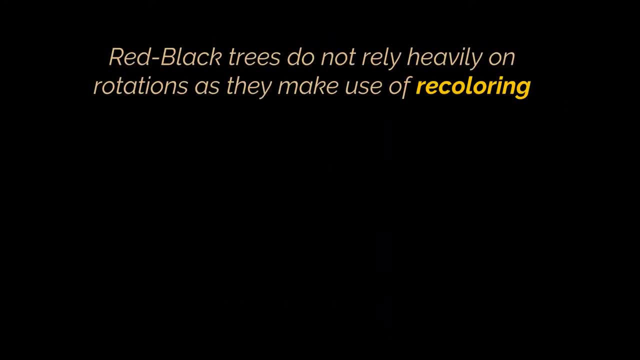 rotations while keeping the tree approximately balanced. Now onto the more serious part. if we are not doing rotations all the time, how are we maintaining the balance of our tree? Well, with the help of recoloring. switching between red-black and black colors can and will help us maintain the balance and the threshold. 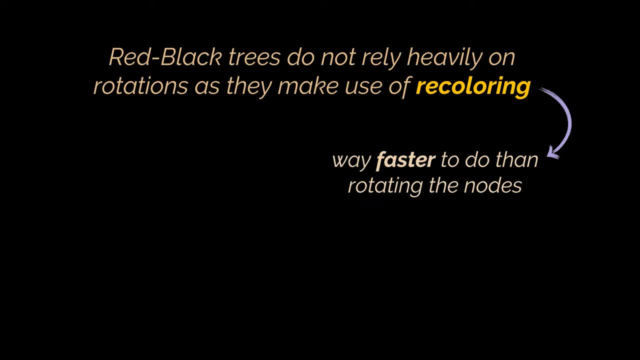 You see, recoloring the nodes of our tree is a way faster operation to do than rotating the nodes and hence will help us reduce the number of operations needed to declare the tree we are dealing with as a valid tree Now, similarly to AVL trees in red-black. 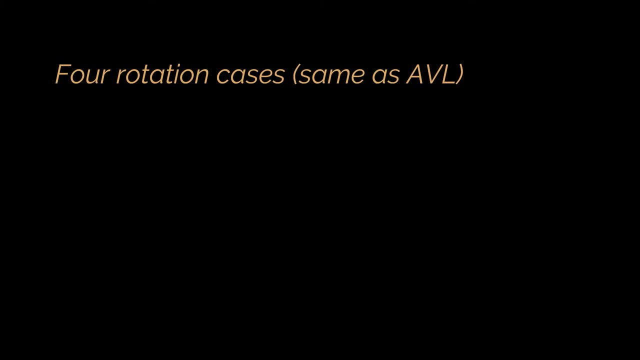 trees. we still have the four rotation situations we discussed, but this time another four will be added to them, and these cases will be resolved only with the help of free coloring the nodes. When will we do rotations and when will we recolor? Well, based on the 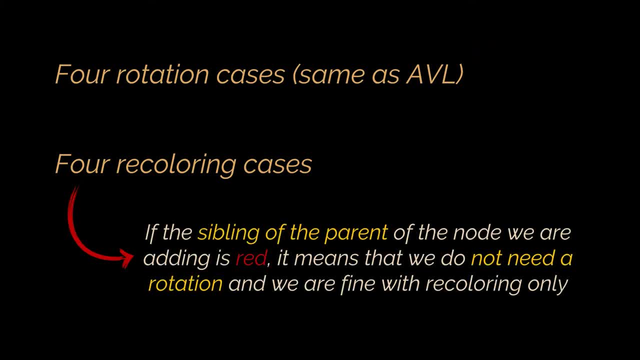 sibling of the parent of the node we just inserted. If the sibling of the parent of the node we are adding is red, which means it is also not null, as null nodes are black, we can safely say that we do not need a rotation and we are fine with recoloring only. However, 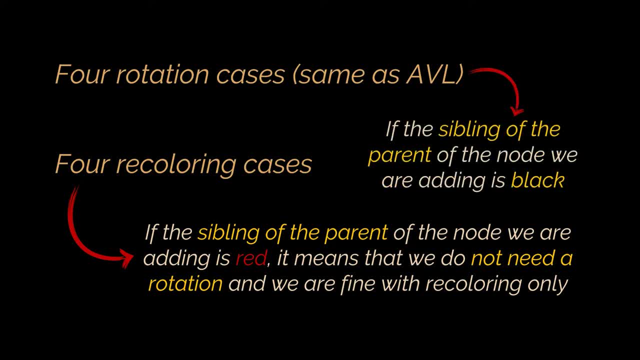 if the parent does not have a sibling or if it has a black sibling. well, we have to go all the way and stick with the four rotation cases we covered in the AVL video. Let's start with the recoloring cases and after we are done, I'll go through the rotation cases briefly. 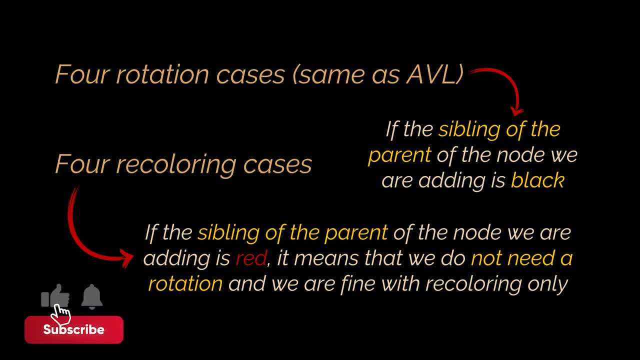 as a refresher to the AVL trees video. But please, if you have no idea what rotations are, make sure to check our latest video, where we cover everything about them in detail. Now, concerning recoloring, we just mentioned that, the parent of the node we are inserting- 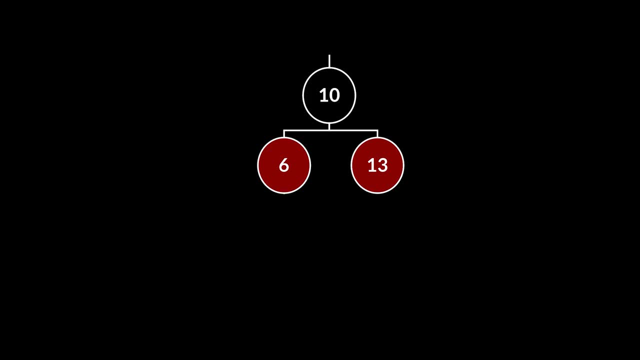 must have a sibling and this sibling must be red. So the tree or subtree you see in front of you could be a very good example of what I just said. Ok, so if we insert this node or node 2. And remember, when a node is inserted it starts off as a red node always. So in our 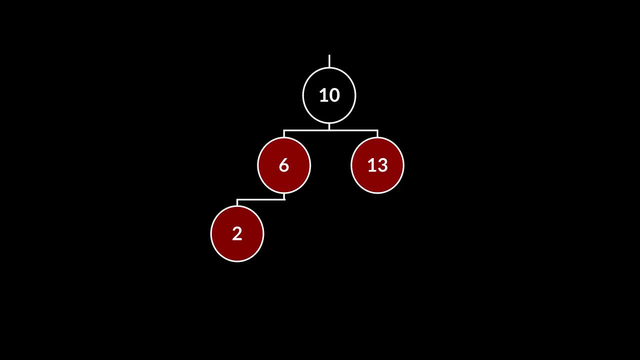 example, we won't need to rotate anything. we just have to recolor the nodes we have, And that is how it's done. The coloring of the existing nodes is simply flipped: What was red becomes black and what was black becomes red, except for the node we just inserted. 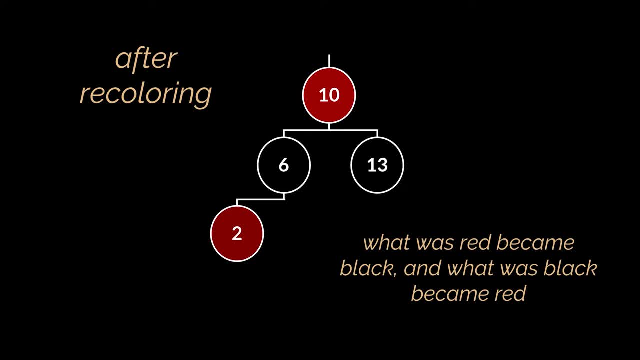 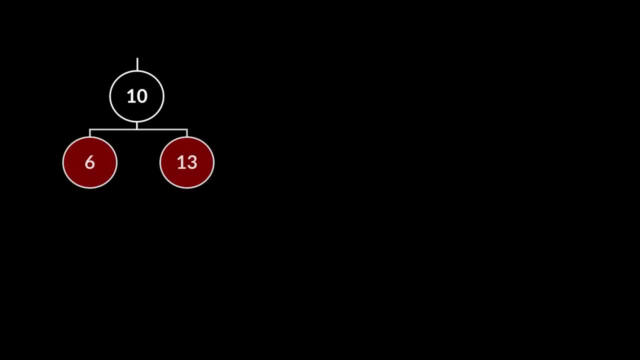 And that's it. No need to do complex rotations or anything. we can just proceed by inserting another node or do any other operation on the tree. The second is basically symmetric to this one with regard to the tree and is also solved by recoloring the same nodes in the same way we recolored the previous ones. 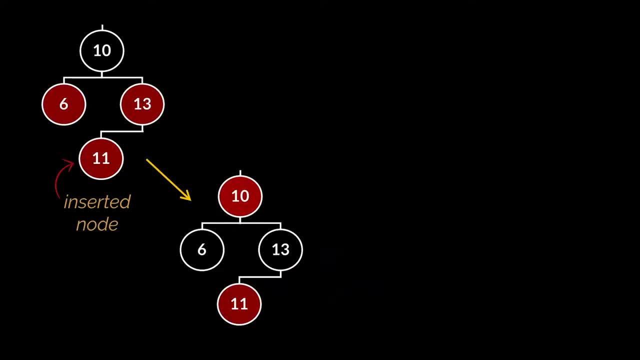 The third and fourth case can now be easily guessed, as they are also symmetric and they require only recoloring, because the sibling of the parent or the uncle of the node we are inserting is a red node. The nodes to recolor are also the parent, the uncle and 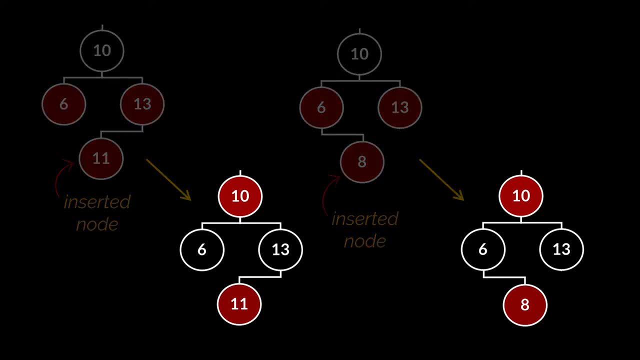 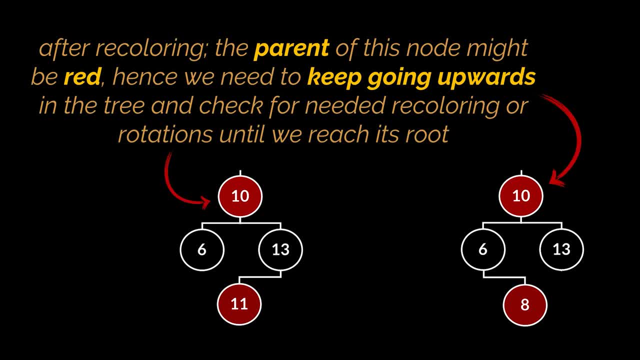 Let's go back to the previous example. Let's go back to recent implementation cases. I need to mention that after recoloring the subtree, you see the parent of its root node might be red. Hence we need to keep going upwards in the tree and check for further needed recoloring. 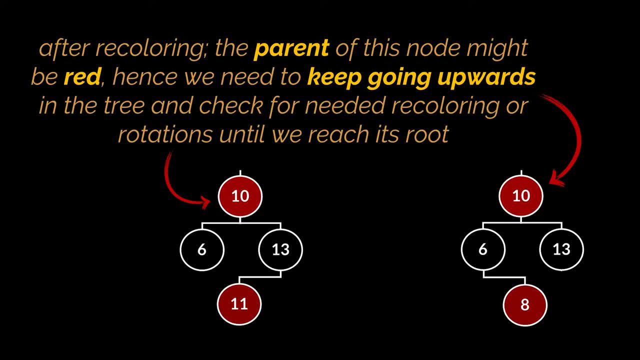 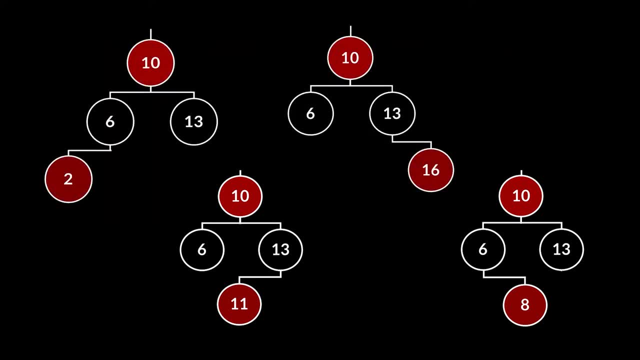 or rotations until we reach the root of the whole tree, And to do this we have to hop to another node in the upper part of the tree. In the recoloring cases we just covered, after recoloring we need to hop to the grandparent. 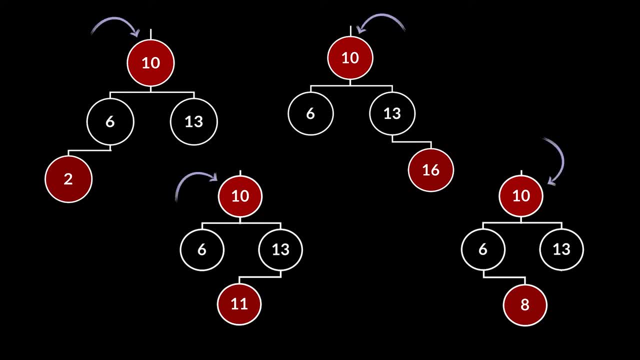 of the node we inserted, which means we need to hop by two nodes and therefore the next node we will be checking is the grandparent checking is the grandparent of the inserted node. We will then keep moving upwards based on the situation we are placed in by the grandparent node and until our tree is declared as a valid. 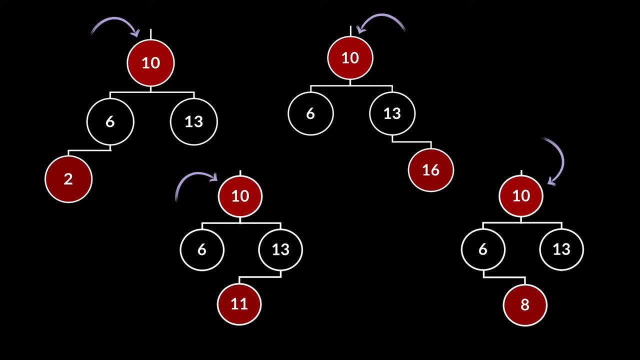 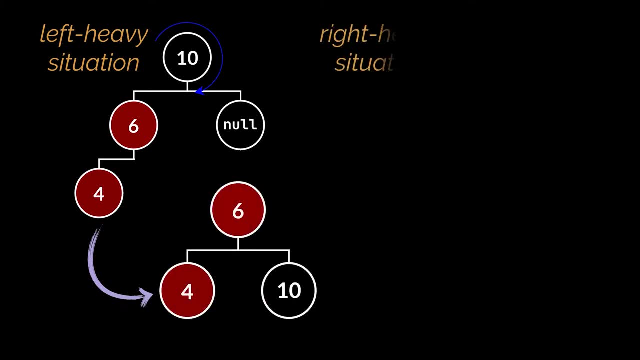 red-black tree. Now let's go over the four rotation cases we previously covered and let's start with the left-heavy and right-heavy situations. These are respectively resolved with a right or a left rotation on the grandparent of the node we inserted, as we saw in the AVL. 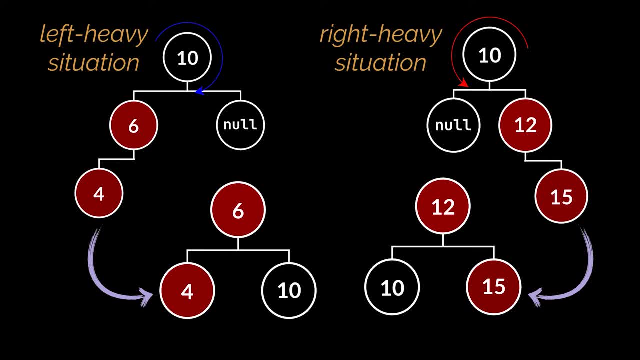 trees video. However, a rotation is applied here only when the uncle of the node we are trying to insert is a black node. Additionally, after rotating, you may have noticed how the trees we obtained do not respect anymore the red-black tree rules we stated at the beginning of the video. 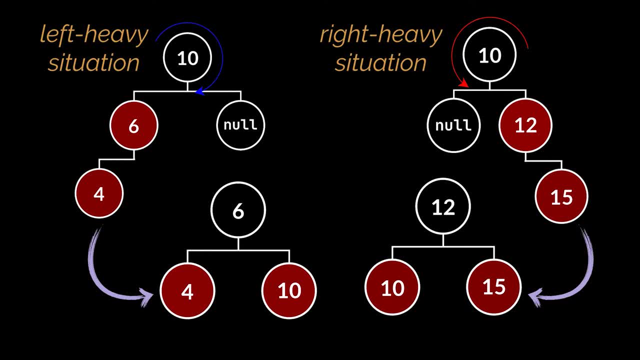 So, on top of rotating, we will need to recolor the parent and the grandparent nodes of the node we inserted. What we also need to take note of is the next node we need to hop onto in our upward tree. scan In both. 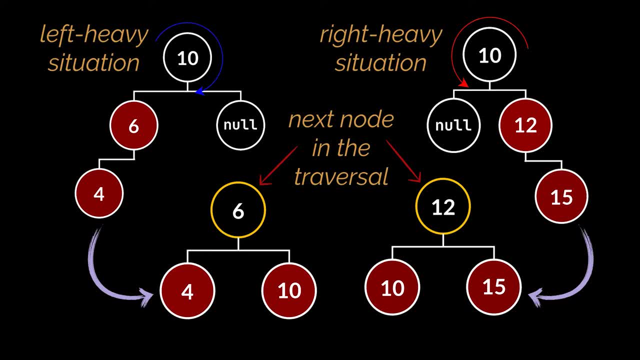 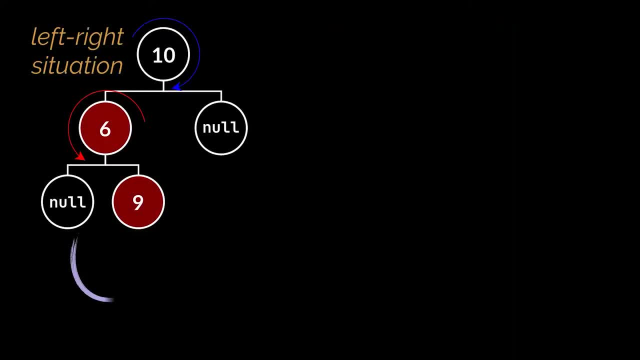 these situations, the parent node is the node we want to check next while traversing the tree in attempt to fix it. The last two remaining situations are the right-left and the left-right situations. These cases are resolved, respectively, with a right rotation on the parent of the. 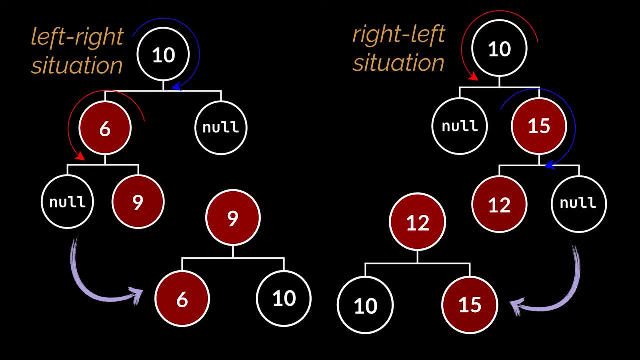 inserted node, followed by a left rotation on its grandparent, and with a left rotation on the parent of the inserted node, followed by a right rotation on its grandparent. The coloring is similar to the previous cases, as the color of the parent and the grandparent are the same, but the 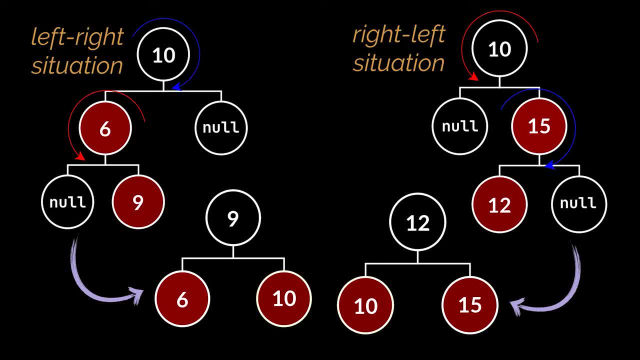 color of the parent and the grandparent of the inserted node needs to be flipped. However, the next node we need to hop onto in our upward tree traversal for these two cases is the old grandparent node and not the parent. Why Let's move on to the implementation And together, while implementing, 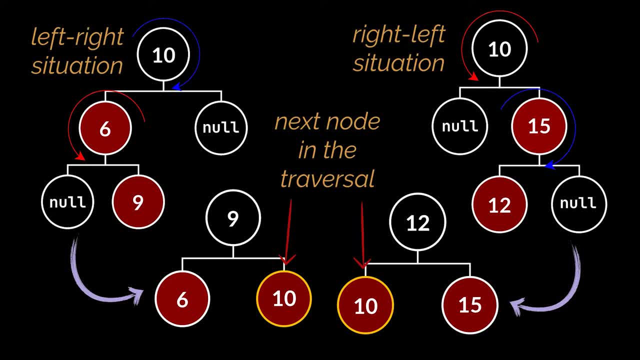 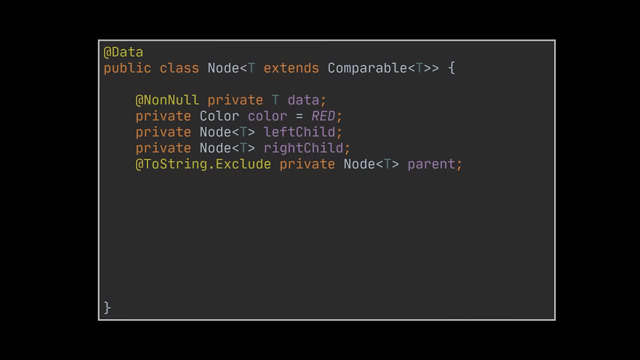 we'll try to answer this and several questions you may still have concerning red-black trees. As usual, we first need to start with the node class For red-black trees. this class has a few extra fields compared to the default or AVL binary search tree. 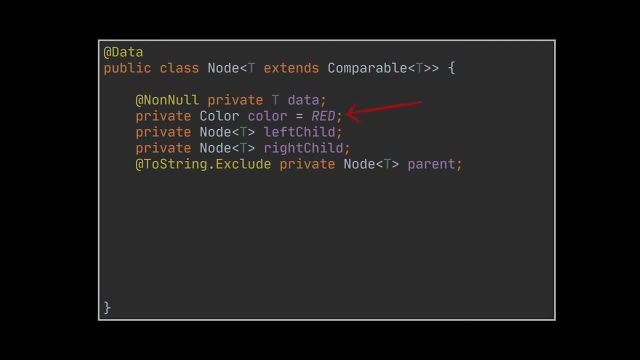 First, in the color field, which represents the color of our node, whether red or black. this field can be an integer, a string, an enum or whatever you prefer. In my case, I chose to use the color class provided by JavaFX, as in a future video, I'll draw the red-black tree. 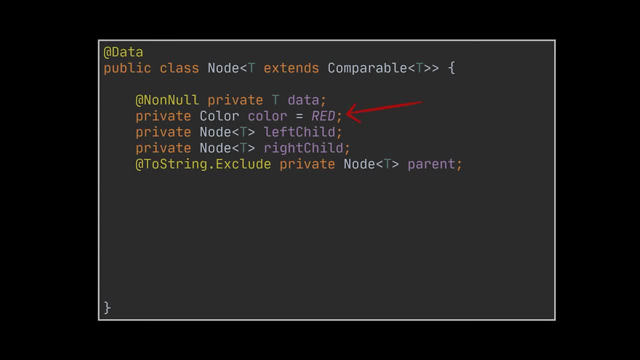 we will create using this class and I'll compare it to the AVL implementation we previously went through. This way, we will be able to visualize the differences between each of the implementations we covered. The next added piece of information is the parent-parent ratio. This is the parent-parent 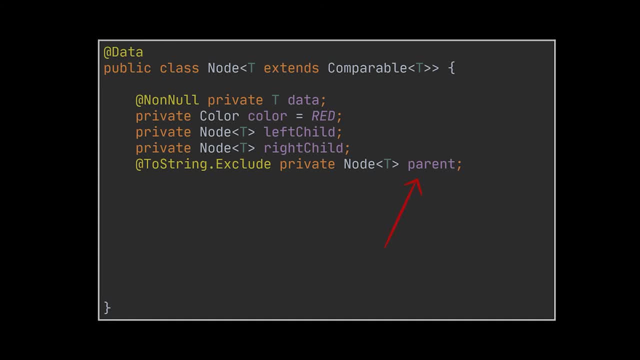 of the node we are creating In red-black trees. we need to keep track of the parent of our nodes, as well as their children, because, if you recall the eight cases discussed, and in order for them to work, we need access not only to the parent of the node, but sometimes to its grandparent. 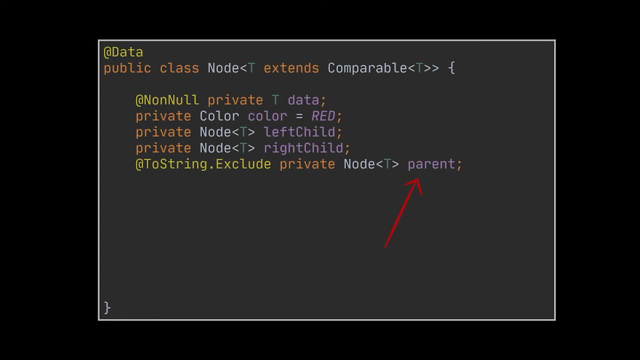 and this is only made possible using the parent field we added Now, after also adding the required Lombok annotations, which will spare us the pain of thinking about getters, setters and constructors. you can stop here and call it a class, However. what I also did was to add a class to the parent of the node, which is the parent of the node. 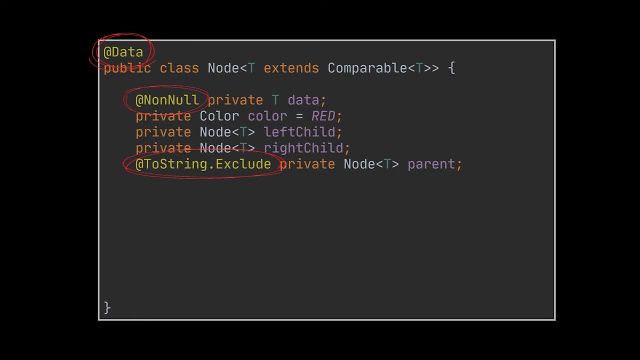 and the parent of the node, which is the parent of the node. The first method was add two extra helper methods: the isLeftChild and flipColor method. These methods will turn out to be very helpful while implementing the recolor and rotate logic. 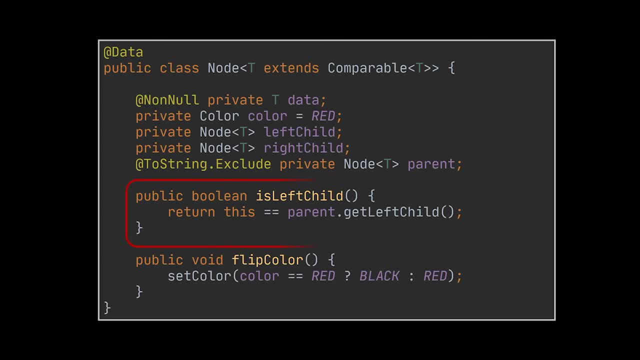 for our red-black tree class. The first one will return true if the node you are calling it from is a left child itself, and if it is a right child it will return false. The second one will just flip the color of the node. So if the node calling this method is a black node, it will make it red. 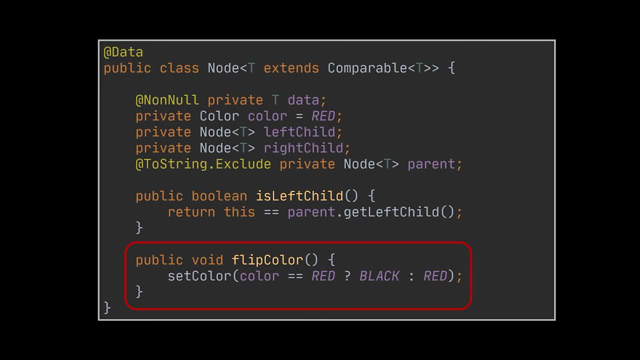 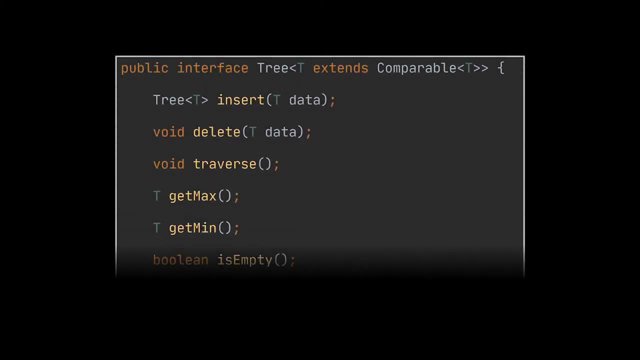 and if it is a red node, it will make it black. These two methods. we can now move to the interface of our implementation, the tree interface. Notice that this interface is exactly the same one we implemented in case of a binary search tree. 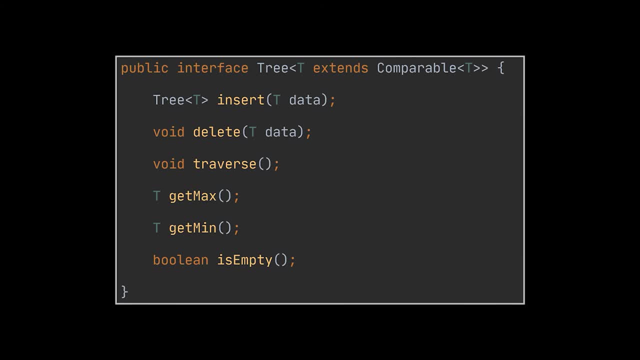 and, in case of the AVL tree, That is why it is called an interface. actually, That is not all, because checking if the tree is empty or not, retrieving the maximum or minimum element from the tree and traversing a tree all have similar implementations to the ones covered in the 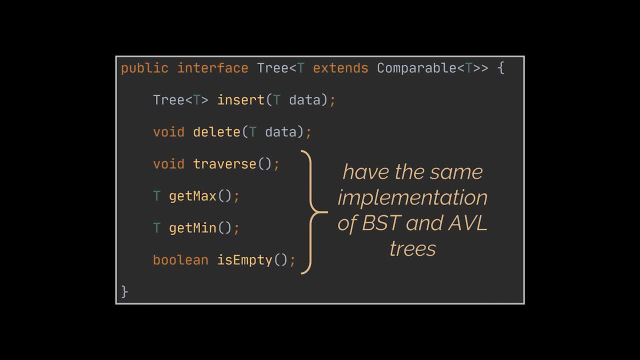 previous videos of this series, the binary search tree and the AVL tree. What we will still have are the insert and delete operations. Let's start by implementing the insert operation. To do that, I will retrieve the insert implementation we already saw in our binary search. 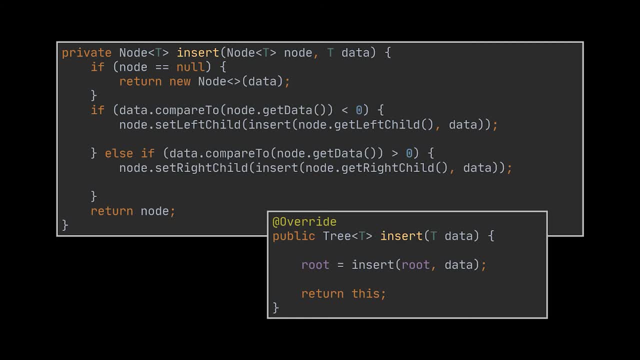 tree and AVL trees video. What we need to do now is adapt this implementation to reflect the requirements of a red-black tree. We previously mentioned that, after the insertion process is done, we need to traverse our tree in an upward manner, starting from the node we inserted until 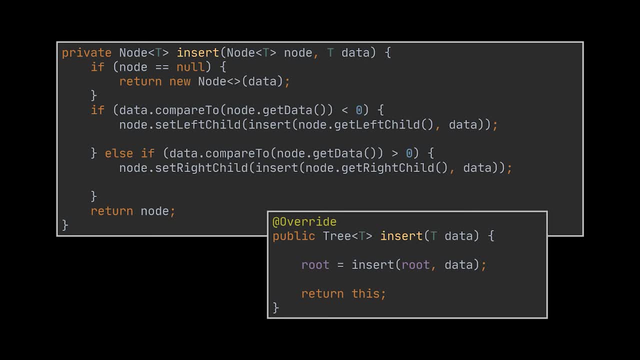 we reach the root in an attempt to recolor or rotate the nodes that fall in any way. So we will do this in any of the eight cases. This was done by calling the recolor and rotate method after the insert recursive calls are completed. However, to be able to do this, we will need 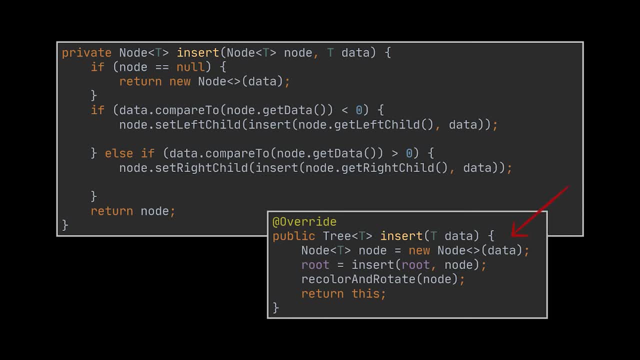 to create the node to insert before invoking the insert recursive call, contrary to what we were previously doing. Therefore, this will require from us to change the signature of the insert method we previously had from taking the raw data to now take the whole. 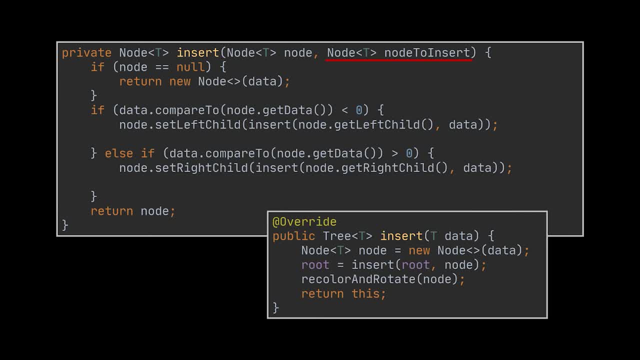 created node as a parameter. So instead of creating and returning a new node in the first if statement we have, we will just return the node provided to the method, and the recursive invocations to the insert method will now take two nodes instead of a. 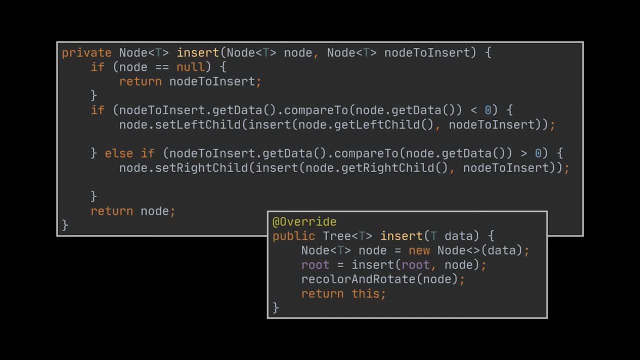 node and a data type. The last thing we need done to adapt this method is assign the parent of the nodes, just as we are assigning their children, in order to avoid null values and null pointer exceptions. This is done by setting the parent of the left or right child, respectively. 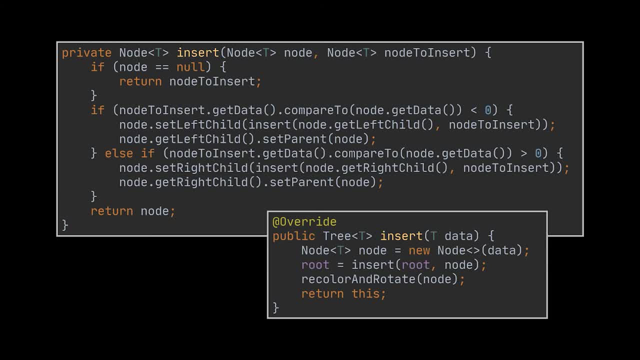 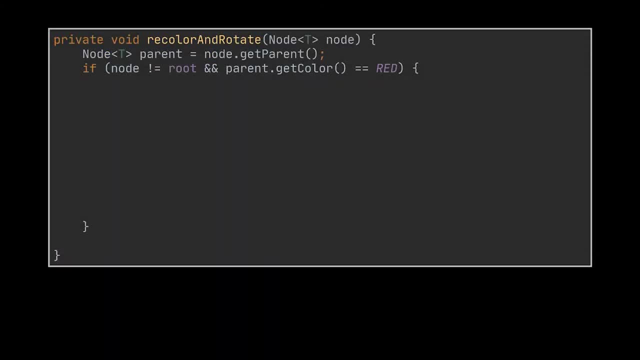 to be the node passed to the method initially. Let's go ahead now and try to implement the recolor and rotate method we just made use of. The first thing we need to do in this method is check if we actually need a recoloring or 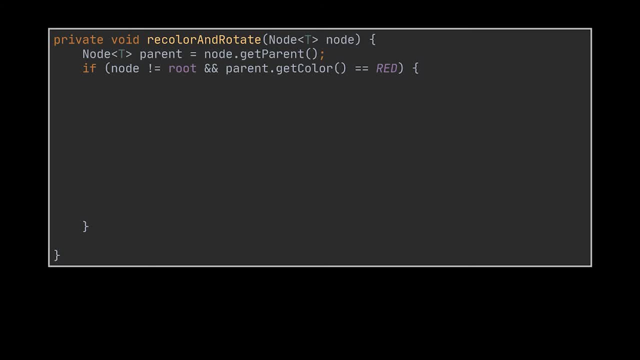 a rotation. I didn't explicitly mention this previously, but if the parent of the node we just inserted is a black node, we most probably didn't violate the red-black tree rules. The red node we just inserted will for sure have both its parent and children. 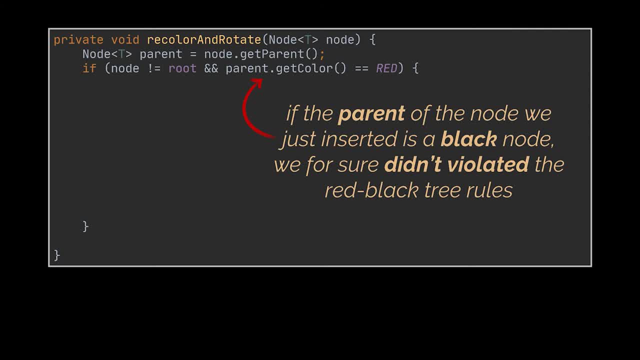 black and the number of black nodes from the root to any null node didn't change as we inserted a red node. So until we reach the root we only need to recolor or rotate. if the parent of the node passed to the method is a red node, This is represented. 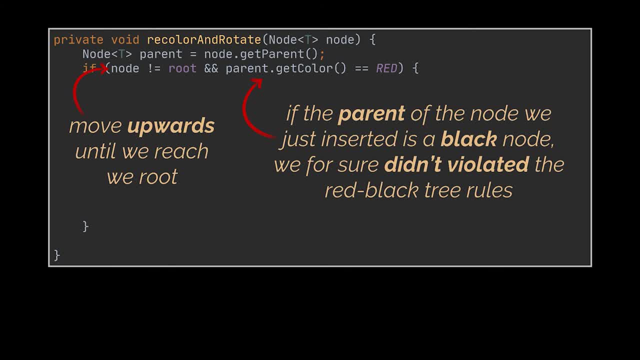 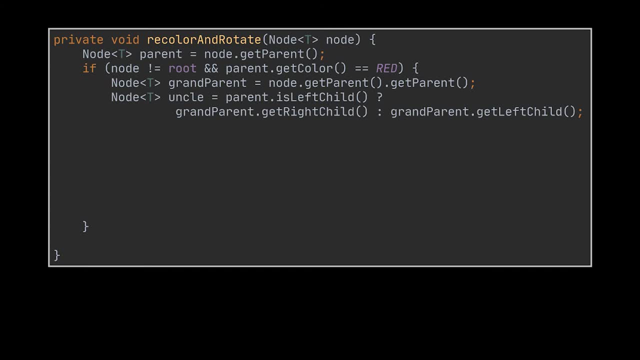 by the if statement you see in front of you. Now, if the parent of the node is indeed a red node, then we have to retrieve the uncle of this node to base our case selection on it. So if the uncle is red, we can stick with recoloring the nodes only. However, if 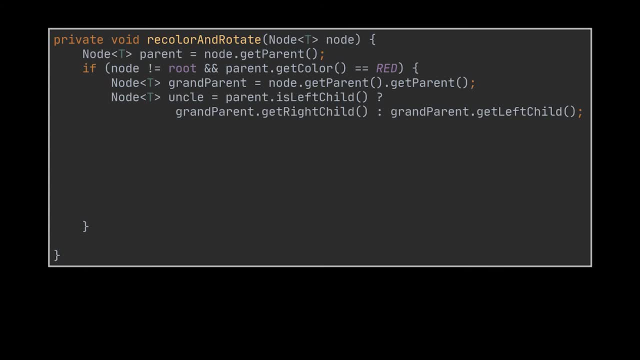 the uncle is a black node, then we will need to rotate the nodes. This logic is represented by the if-else conditions you can see. So if the uncle is present and is a red node, then we have to implement the recoloring logic. If the uncle is a black, 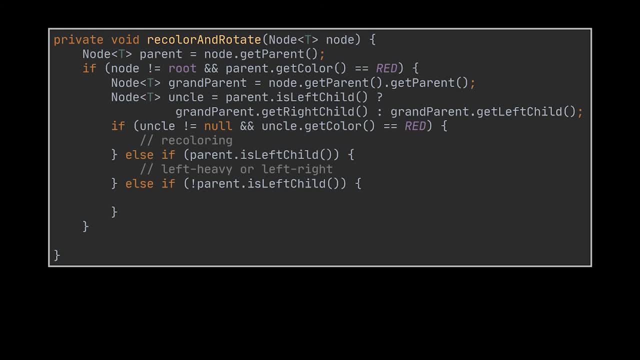 node and a left child, then we have to deal with either the left-heavy or left-right situation And finally, if the uncle is a black-right child, then we have to cover the right-heavy or right-left situations. For the recoloring part, we stated that we 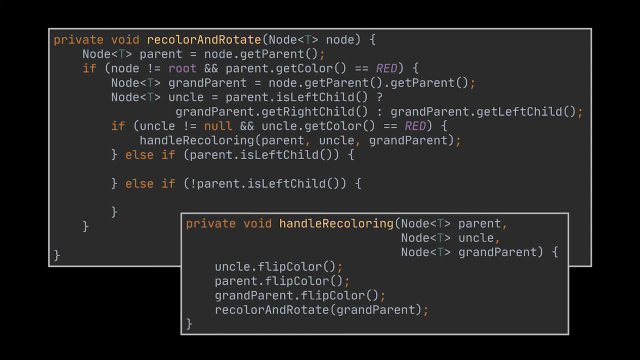 will need to flip the colors of the uncle, the parent and grandparent nodes. Then, while moving in our upward tree traversal, we will move to the grandparent node, and that is what this recursive call to the recolor and rotate method is here for. This call will 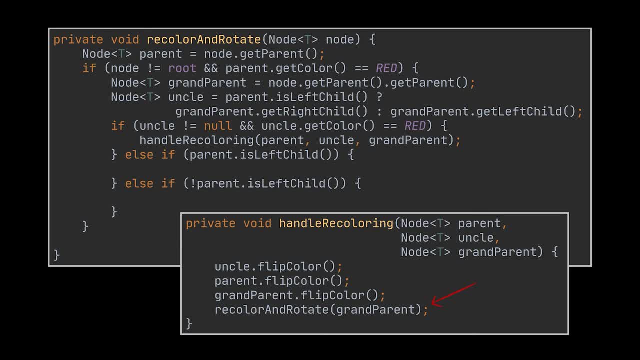 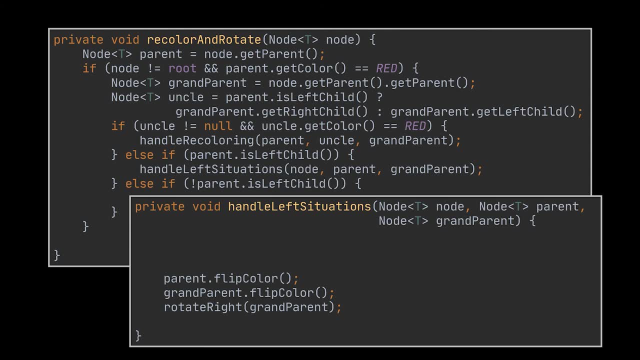 allow us to move in an upwards manner from the node we inserted to its grandparent node. Next, if we are in a left-heavy situation, a right rotation is needed on the grandparent node of the node we inserted, as well as a recoloring of both the parent and grandparent. 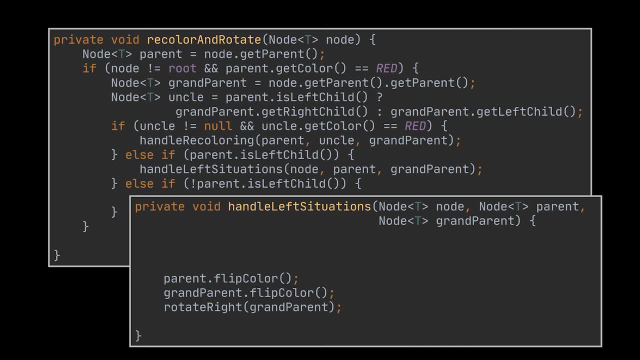 nodes. as we previously mentioned, This was done using the flip-color method already implemented In the heavy situations. unlike recoloring, we will need to move to the parent node next, and this is done by invoking recursively the same method as you can see in front of you. Now for the left-right situation. if the 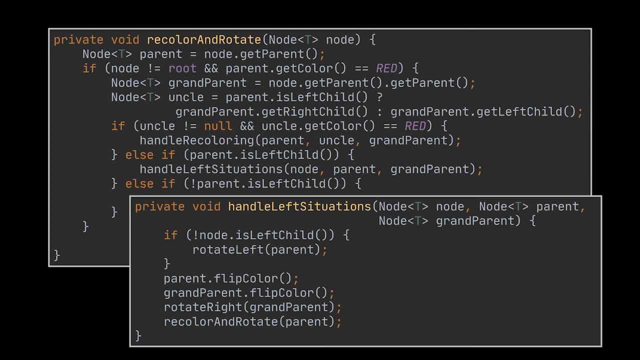 node we are inserting is a right and not a left child, then a left rotation is required on the parent of the inserted node, followed up by the right rotation we just wrote down on the grandparent of the node itself. However, for this situation, we have to hop to the 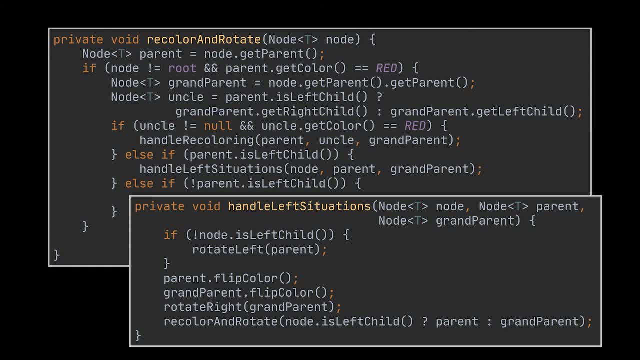 grandparent node in our traversal and not the parent node. This was tackled here using the ternary expression you can see, And basically the same condition check used in the previous if statement. Concerning the right-heavy and right-left situations, they are symmetric to what we 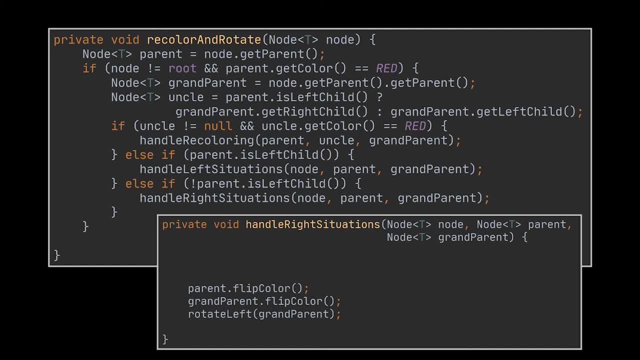 just covered. So in the case of a right-heavy situation, on top of recoloring both the parent and grandparent of the inserted node, a left rotation is needed on the grandparent. Moreover, in case of a right-left rotation, we have to do a right rotation first on the parent. 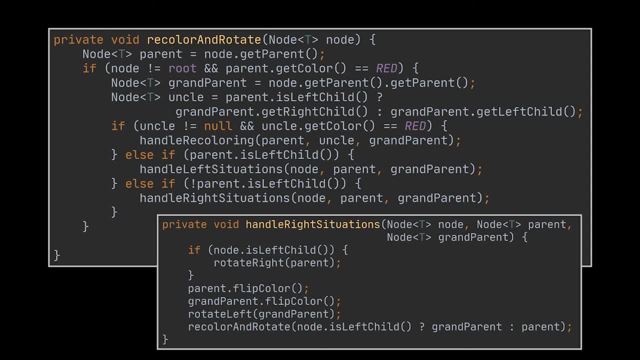 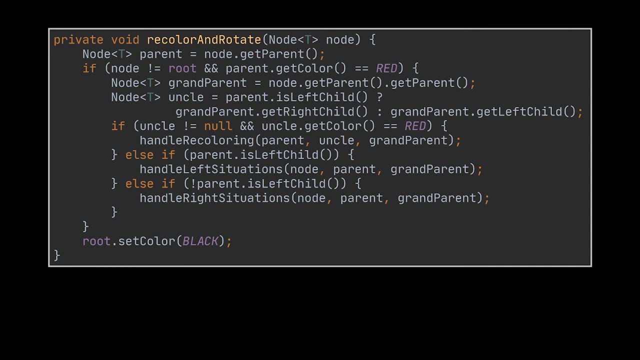 followed by a left rotation we just added. The hopping is pretty similar to what we just saw and uses the same condition of the if statement we have. The last thing we need to do to complete this method is explicitly color the root node as black, so that the first condition of the red-black tree after we finish the traversal 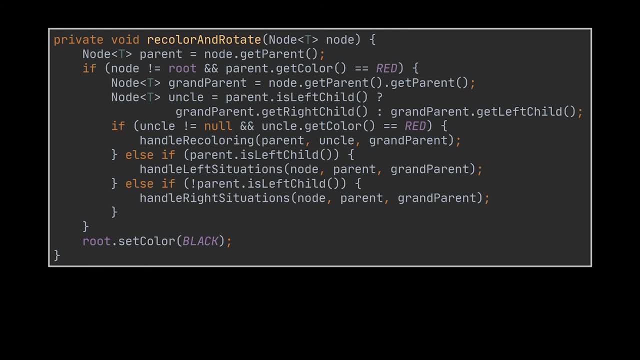 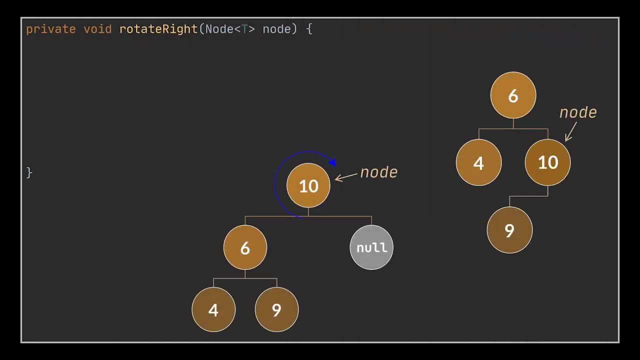 is met. Now that we are done with the implementation of the recolor and rotate method, let's go ahead and apply the required modifications on the previously implemented rotate-right and rotate-left methods. Let's suppose that's the initial tree we have and want to perform a right rotation on it. 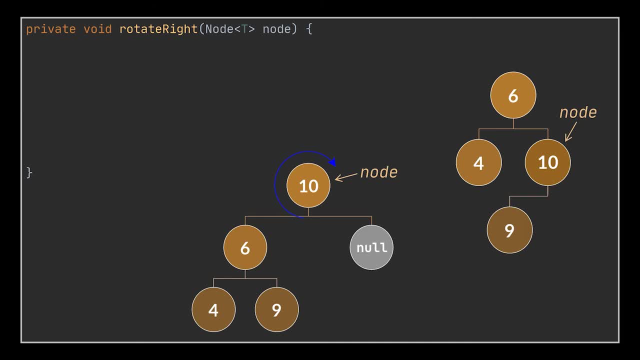 Next to it you can see the result of this rotation, what the tree should look like after the rotation is performed. The only difference between this implementation and the avl-tree one is that here we need to update the parent fields also, and not only the children. 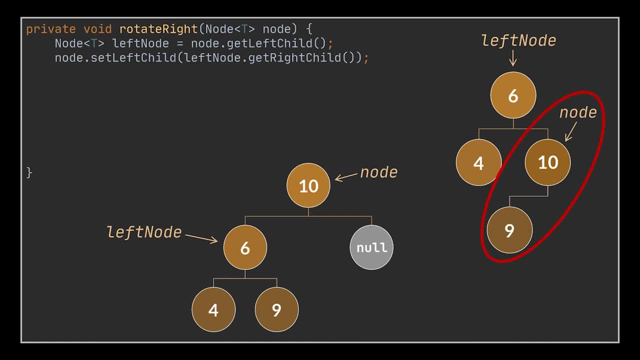 So, as we previously did, we will first start by setting the right child of our left node to be the left child of our root or the node passed to the method. So in our example here we are setting the 9 to be the right child of 10.. 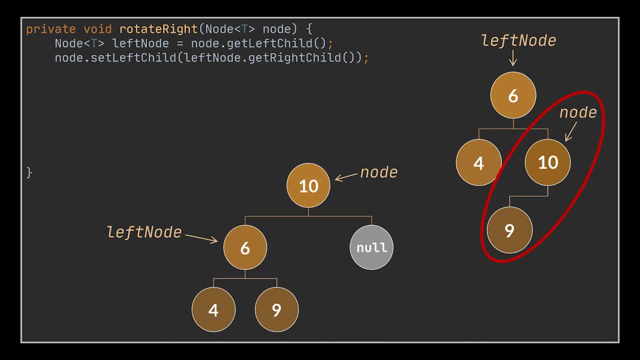 Now, in some cases, especially when we are facing a left-heavy situation, we need to modify the right child of our left node to be the left child of 10.. In this situation, this node is null and to avoid null pointer exceptions, what we have 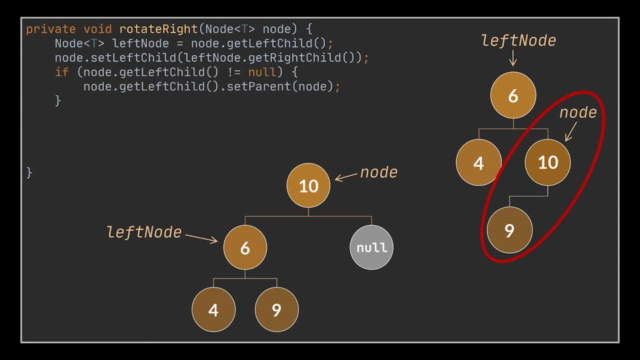 to do is check if that's the case or not. If this node is not null, then what we have to do is set its parent to be the node variable. So in our example, we set the node 10 to be the parent of node 9, which is similar to. 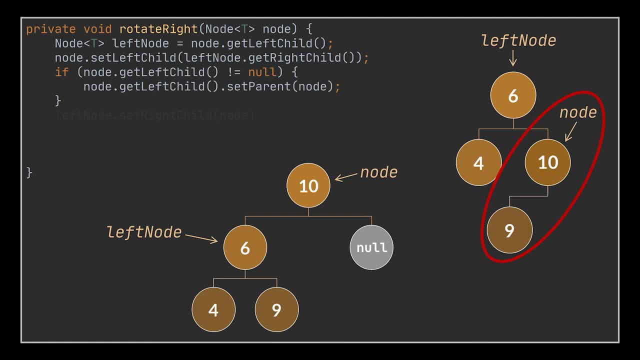 what we are expecting in the results. The next thing we need to do is modify the right child of our left node variable to be the node passed to the method and it is now located to its right. So 10 will be the right child of 6.. 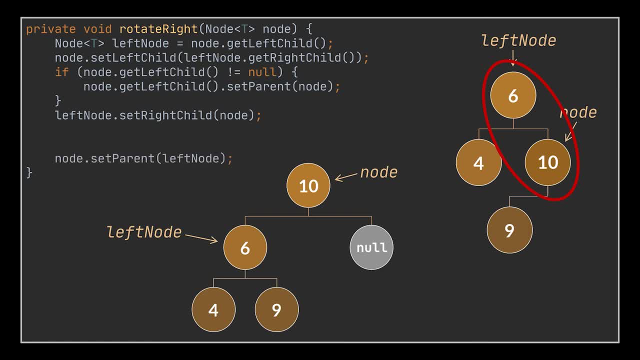 And, consequently, the left node will now be the parent of our old root, and the parent of our old root, or the node passed to the method, will now be the parent of the left node. However, before setting the left node as the parent of the node variable, we have to do: 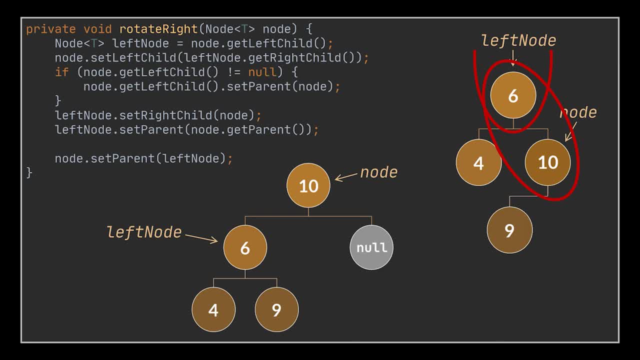 one last thing before this information is lost. What information? Well, we still haven't updated the children of the parent of the node variable. You see, the parent of node 6 is now pointing to whatever the parent of 10 was, but the. 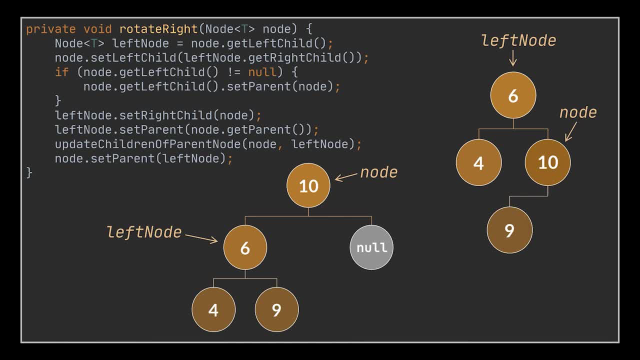 parent of 10 isn't pointing to the parent of 10.. It is still pointing to node 10.. And while traversing the tree, if this reference is not updated, everything we did would have been in vain. So let's implement this tiny helper method together. 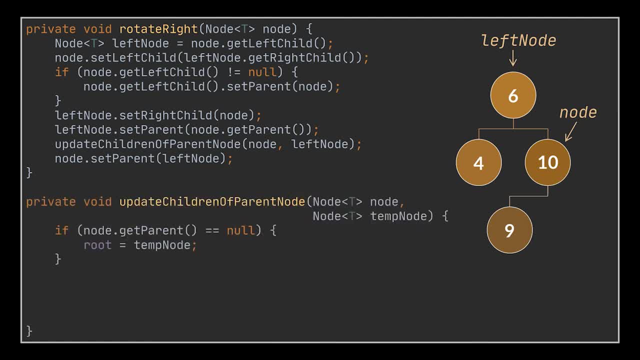 Inside this method we have to first check if the parent of the old root was null, because if that is the case, then this node was the root of the whole tree and node 6, in our case, should become the root node of the tree. 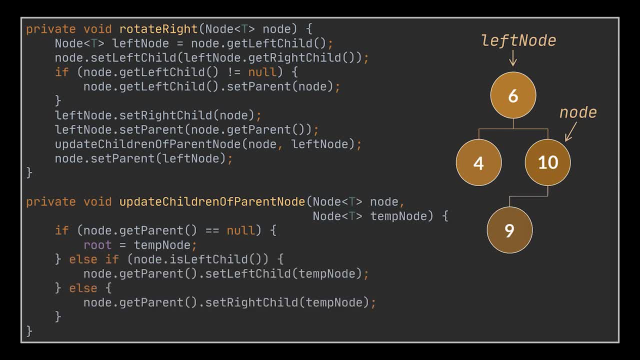 However, if this node was a left or right child, then we have to set the left node to be the left or right child of the tree. With this last addition, the rotateRight method is now complete. Concerning the rotateLeft method, it should be pretty straight forward now as it is symmetric. 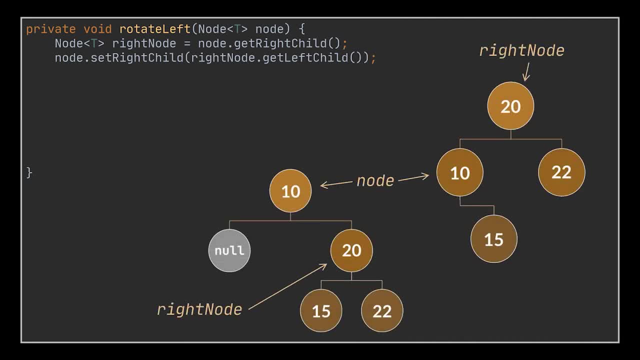 to what we just implemented in regard to the tree. So we have to start by setting the right child of the node passed to the method to be the left child of our right node variable and then proceed by checking if this node is a null node or no and if it isn't, we update its parent accordingly. 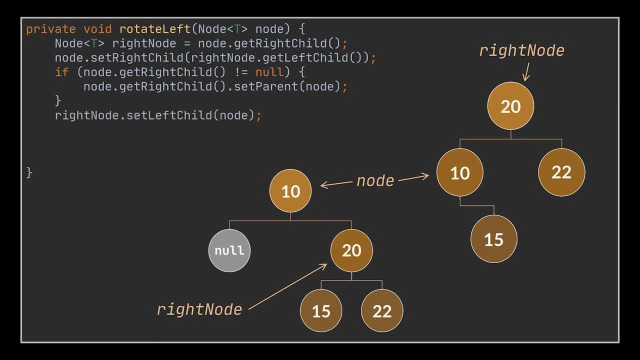 The next thing we need to do is update the left child of the parent of the tree to be the left child of our right node variable and then proceed by checking if this node is a null node or no and consequently, similarly to the rotateRight method, we have to update: 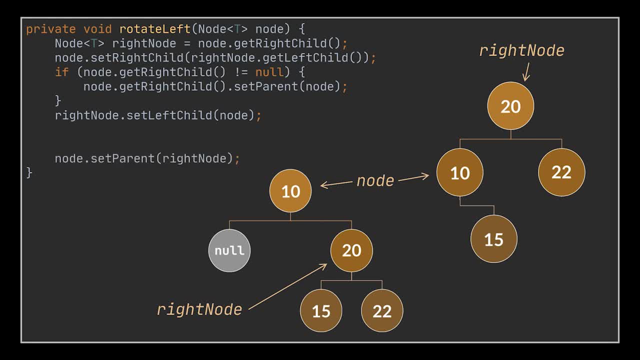 the parent of the node passed to the method, the parent of the right node and the children of the parent node of the whole tree or subtree. we are trying to rotate. To do this final step, we can reuse the helper method we implemented a minute ago. 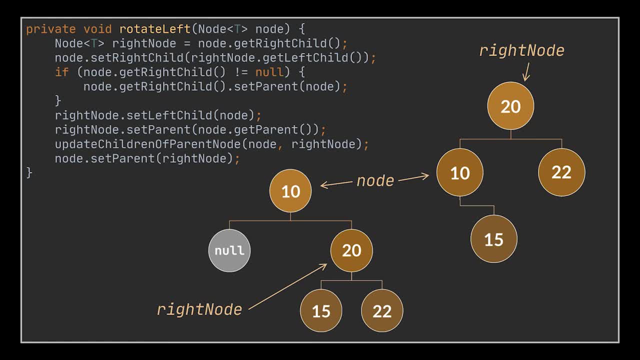 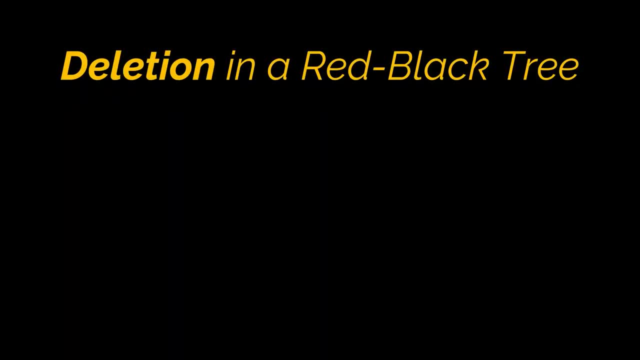 With this, we finalize the implementation of the rotateLeft method and, with it, the insert operation. Now, regarding the delete operation, I won't go through the detailed implementation, as the video is already a bit lengthy as it is. However, if you would like me to do so, hit me up in the comments down below and let me 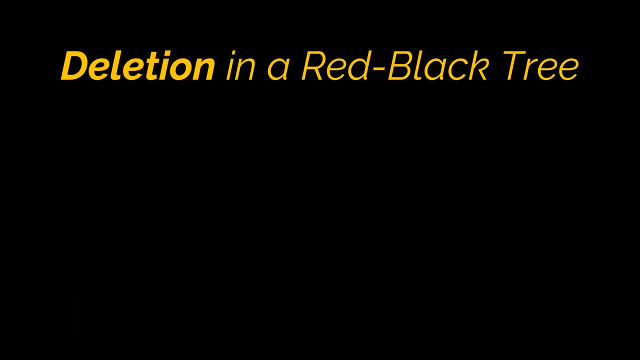 know your thoughts and I for sure will make it happen. So, to delete an element from the red-black tree, we have the same three scenarios we previously covered, which are deleting a leaf node, a node with a single child or a node. 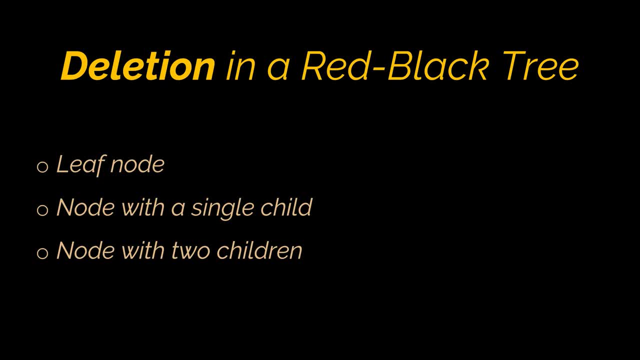 with two children. All these scenarios follow the same solutions discussed in earlier videos. Additionally, after deleting, just like after inserting, we can delete the left child of the tree. By doing so, we have to fix our tree as it may have violated the red-black tree requirements.